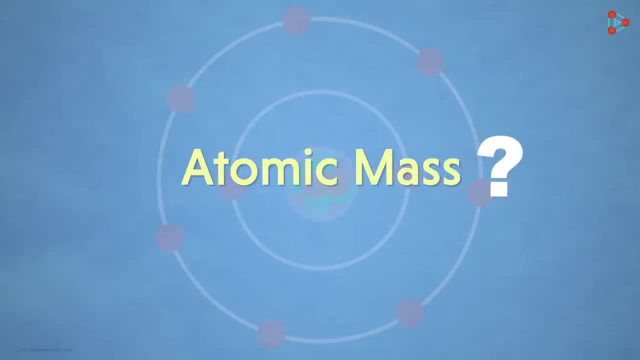 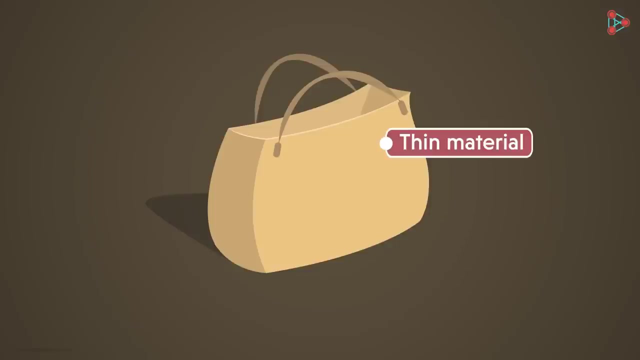 Now, on similar lines, can you tell me what atomic mass could be? Yes, it simply means the mass of an atom. But how does it get determined? Imagine we have a bag which is made up of extremely thin material, So thin that it almost does not have any mass of its own. 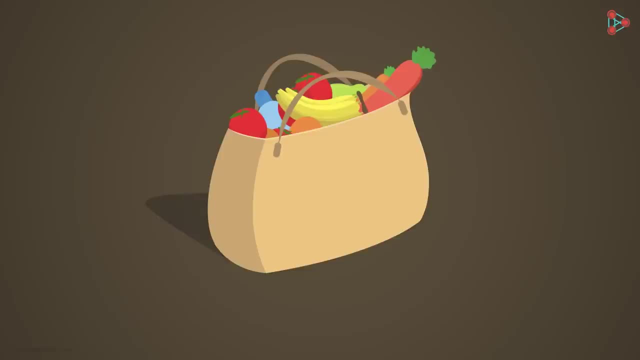 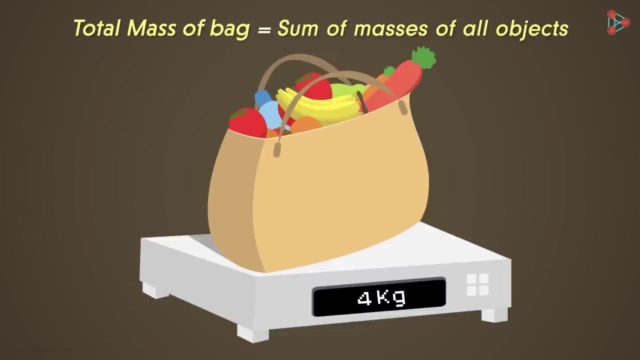 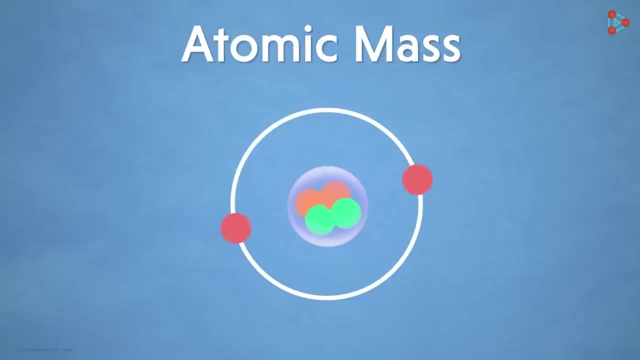 Now we fill this bag with some stuff inside. If this bag is placed on a weighing scale, then can we say that the total mass of the bag will be the sum of the mass of all the objects inside it. Absolutely Similarly, the mass of an atom can be calculated with the help of the subatomic particles in 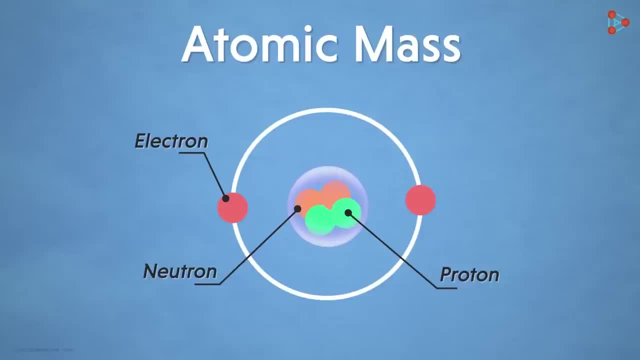 it. But we know that, among all the subatomic particles, electrons have negligible mass, That is, they are considered to be almost weightless. So what are we left with? Yes, we have both protons and neutrons in the nucleus. 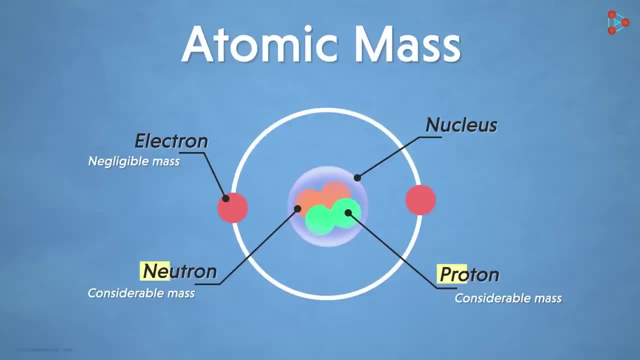 And these two do have some amount of mass is what we know. Now tell me one thing: which among these two particles should be considered? Shall we consider only the mass of protons or only the neutrons, Or both together? Well, since both have a significant amount of mass, we will consider the mass of both. 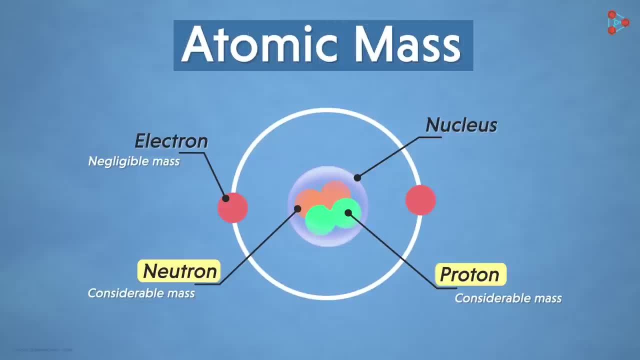 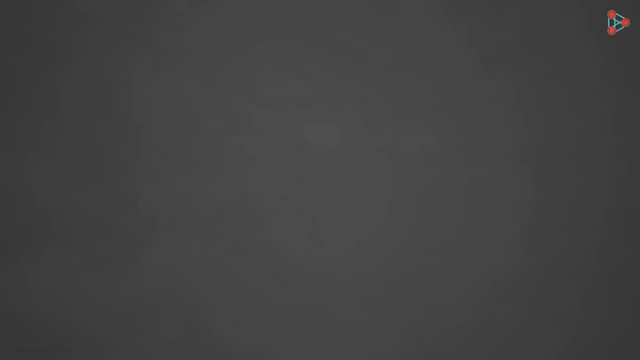 together. Hence, the atomic mass is defined as the total number of protons and neutrons present inside the nucleus of the atom. It is also referred to as the mass number. Let us take a simple example. In case of a simple element like fluorine, we find that there are 9 protons and 10 neutrons. 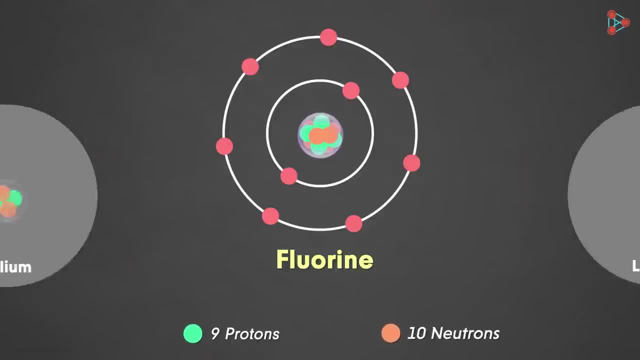 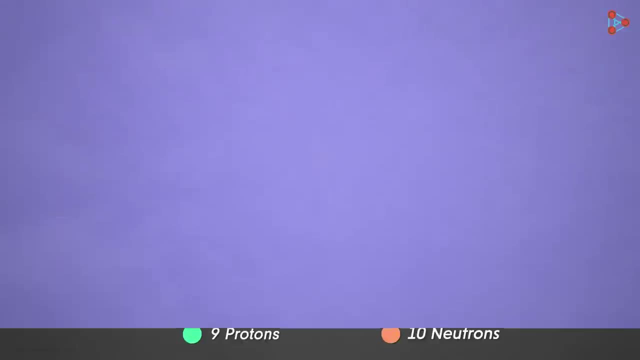 in the nucleus? Wait a second. We have always come across cases where the atomic nucleus has an equal number of protons and neutrons, So how is it that the number of neutrons is more? Well, Tell me, Does the presence of additional neutrons really bother the atom? 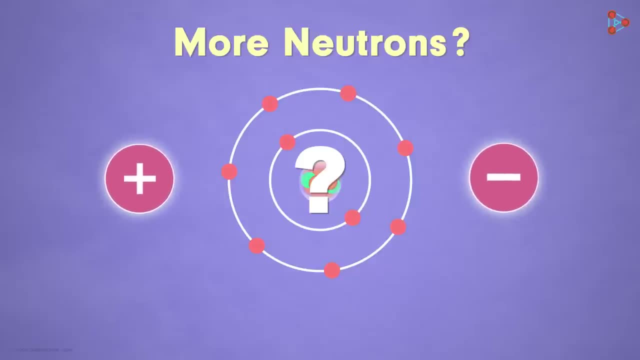 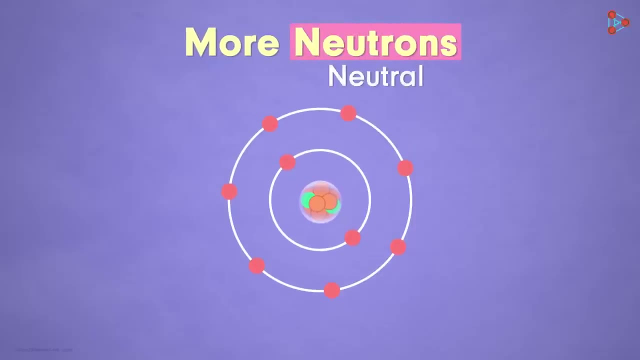 Does the charge of the atom increase or decrease? Absolutely not. That's because they are neutral. Then why should an extra neutron bother us? So, coming back to the atomic mass of fluorine, we have 9 protons and 10 neutrons.